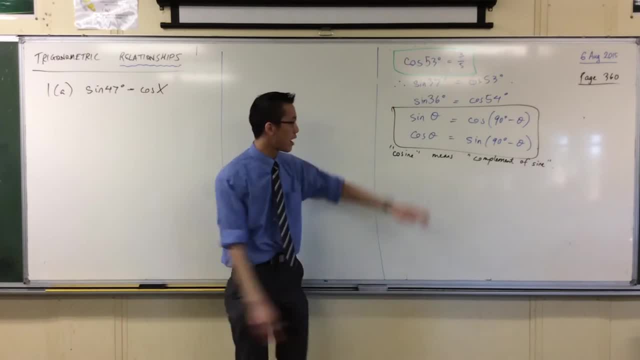 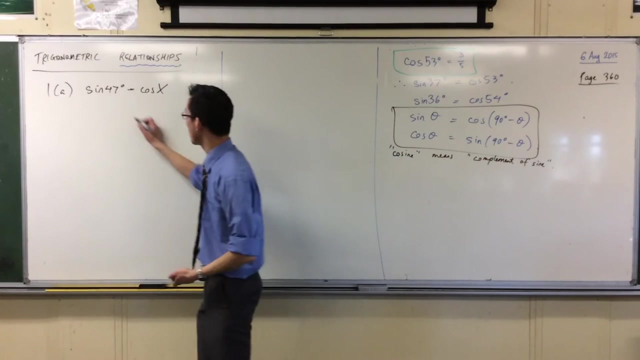 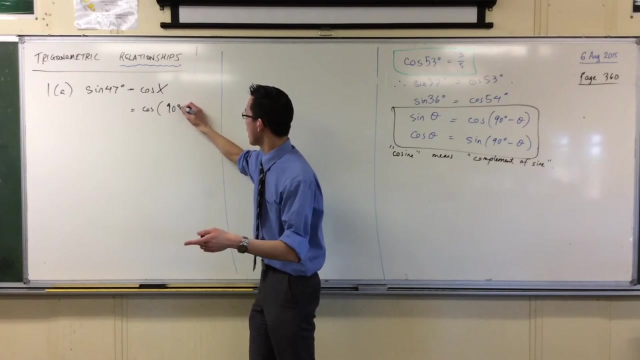 So, looking at this, can you see? this more or less matches what we concluded when we were trying to generalize this pattern, right, trying to make it true for any angle, right? so sine of some angle- there we go, there's my some angle- is cosine of some other related angle, right? so here's what I'm going to write. sine of 47, that's my theta, right, is going to be cos of good. the complement 90. take away 47, there's my complement, okay, which is, I mean you could reach me a calculator. 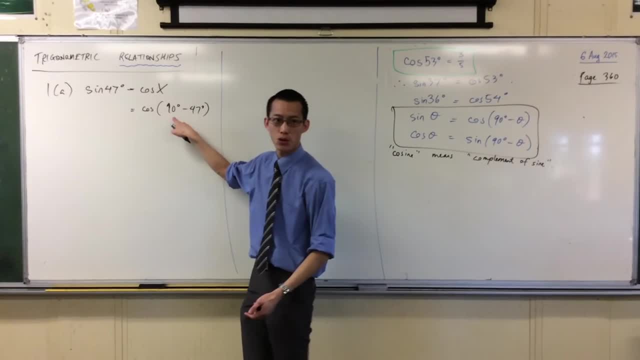 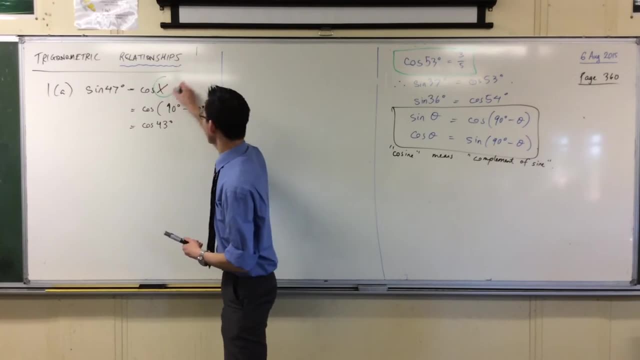 but it's simple enough, right, 47 is going to match up to 43,. okay, so there you go. wasn't very difficult, was it? X is 43, that's not hard. okay, move on down to question 3, it starts to get a little trickier, question 3.. 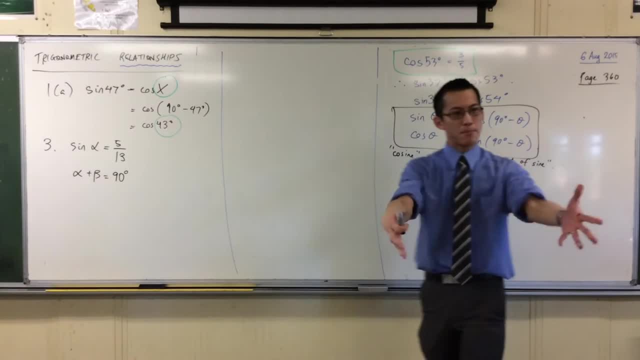 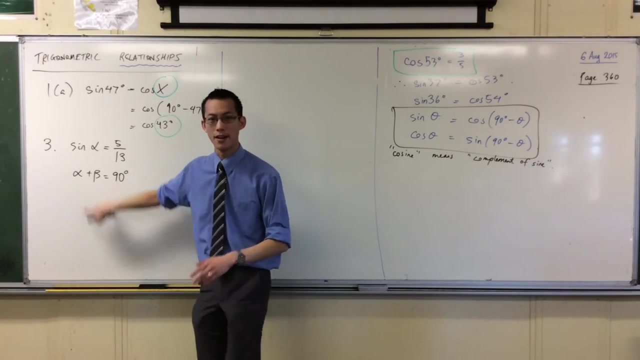 Okay, they present you some information. right, by the way, that's an alpha, that's a beta B with a tail on it, which Greek? that's why we say alphabet anyway, if sine alpha is equal to that and they tell you this relationship between alpha and beta, in other words, they are complementary. you see that. 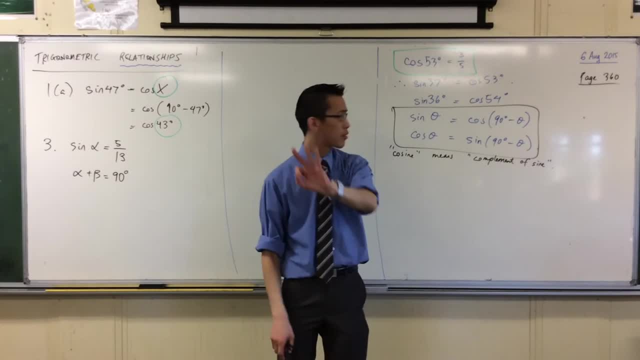 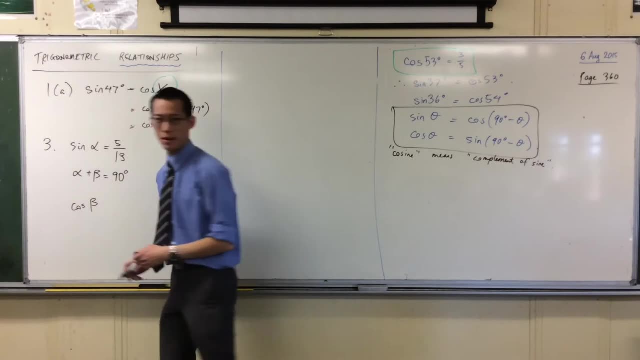 They're both out to 90, it's this kind of situation, right? they ask for three things. they want cos beta, cos alpha, sine beta. okay, so let's start here. cos beta? Now, all I know about these two angles. 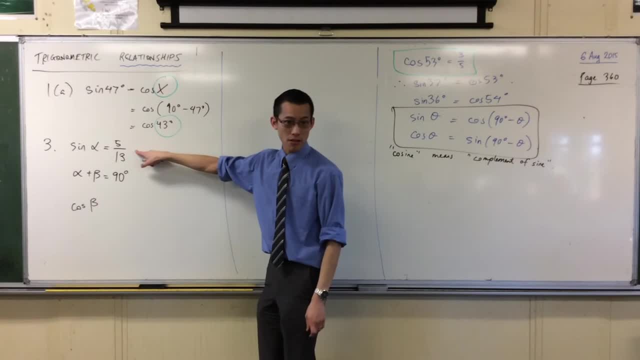 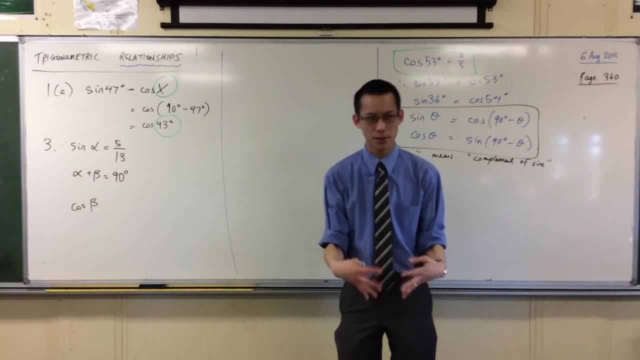 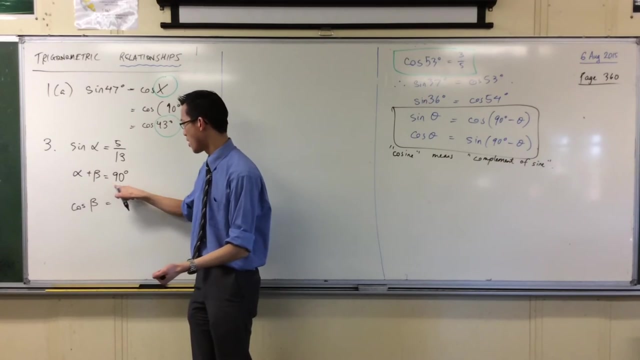 apart from the fact that they are complementary, is I know this, So I can get this in terms of this if I use this relationship. So in other words, I'm trying to sort of assemble a jigsaw here. So cos beta? I can see that beta is 90. take away alpha. 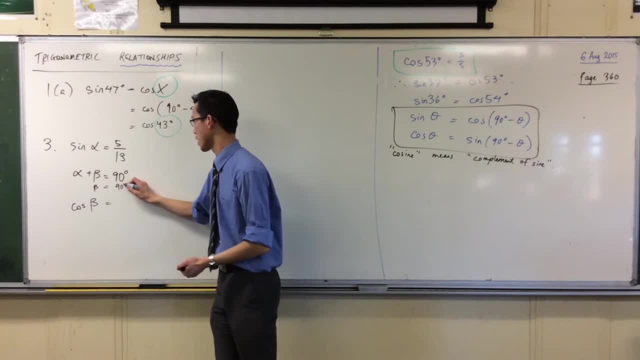 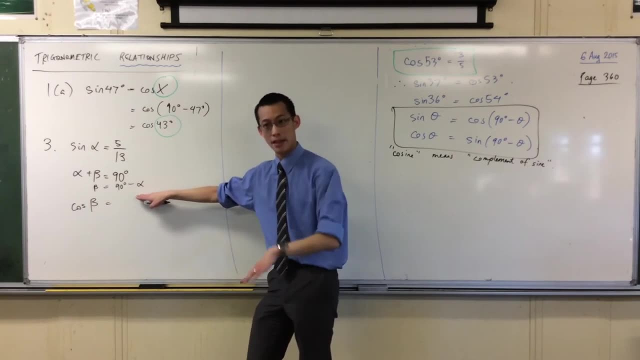 Do you see that? Let me write it in here. I'm just going to take away alpha from both sides. That gives me that. So everywhere I see beta, I could substitute out for 90 degrees minus alpha. They're the same thing. 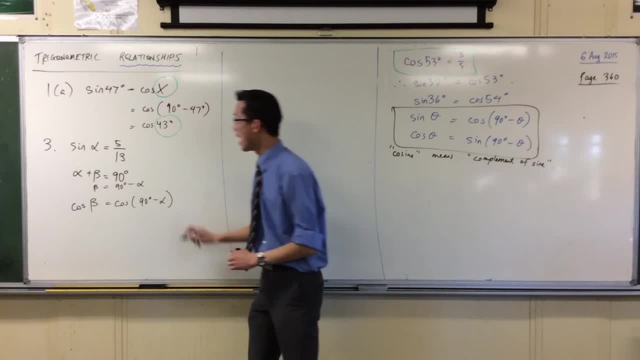 So that's cos of 90 degrees minus alpha. We just took advantage of this relationship, didn't we? It's right here. It's equal to, that's the complement of alpha. So I can say that's sine of alpha, which of course you know. 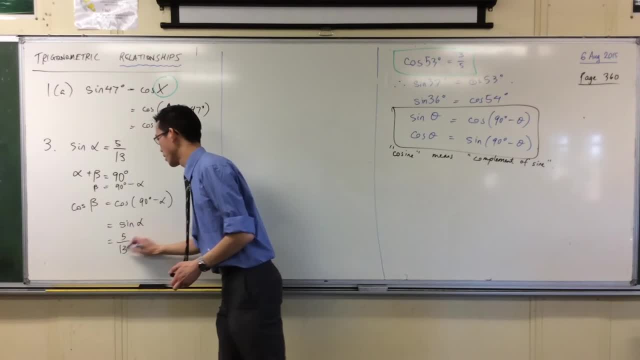 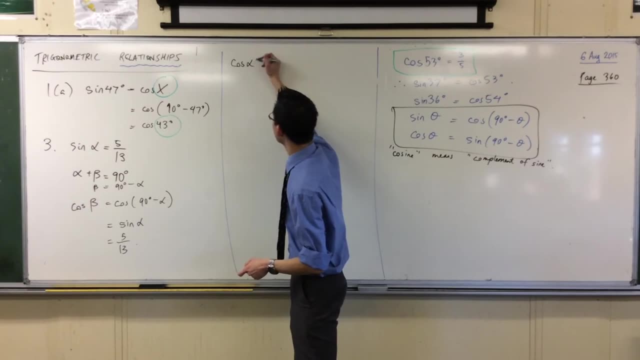 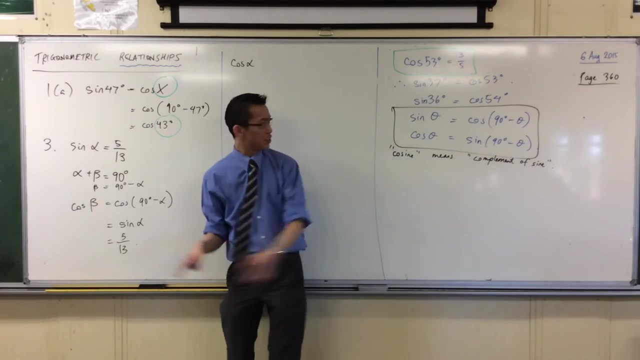 You just got told from the beginning That's 5 over 5.. That's a 13.. Now, if I go to the next one, they want cos alpha, Cos alpha. This is a bit sneakier, You think? hmm, I've already used up my relationship. 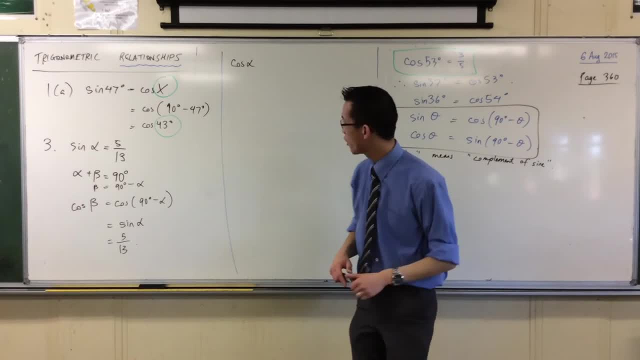 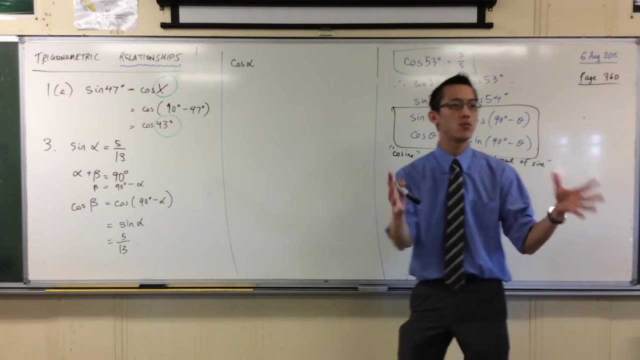 that I knew here before. So now, what direction do I go in? Think back. I'll ask you again: When we first met sine and cosine and tan, where did we meet them? In what kind of shape? We met them in right angle. 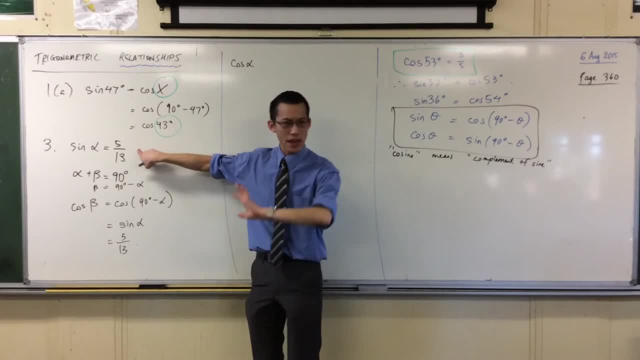 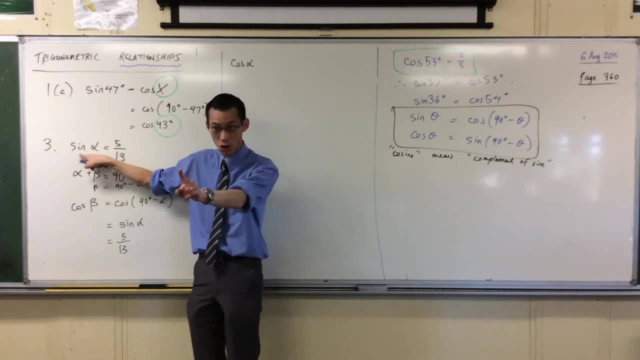 Right angle triangles, Right angle triangles. So this, even though I'm giving you a picture, this implies a picture. It implies a picture where there's a ratio between two sides. You know which two they are, And that's the ratio. 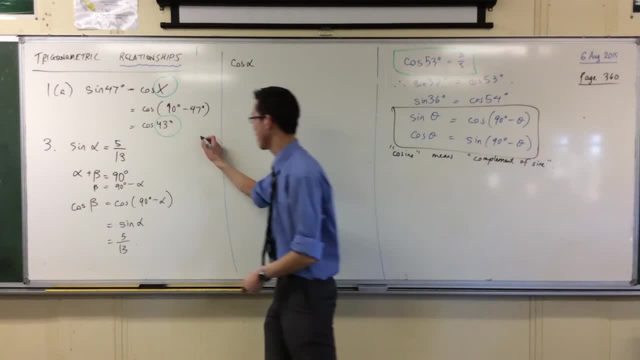 So if a picture is implied, give them a picture. Here we go. Here's my right angle triangle. If I've got alpha and beta being complementary, I'm going to put alpha here and beta here, Because those two angles are going to add to 90.. 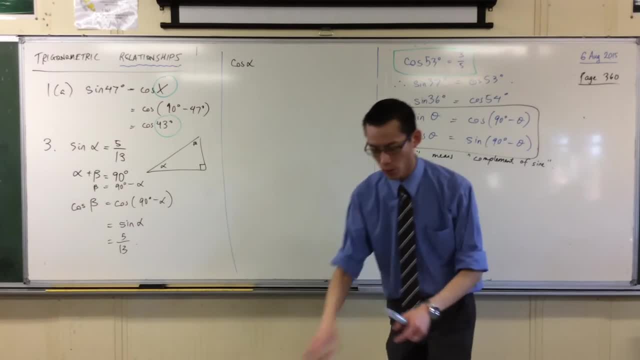 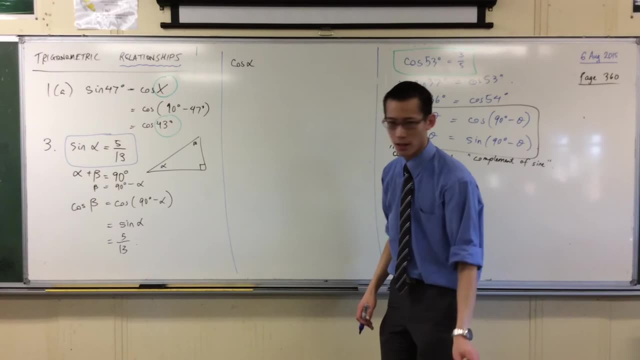 Add to 90. Now sine alpha equals 5 over 13.. Let's take this and try and put that data onto our diagram. Sine is which relationship? again Opposite over hypotenuse. Opposite over hypotenuse. 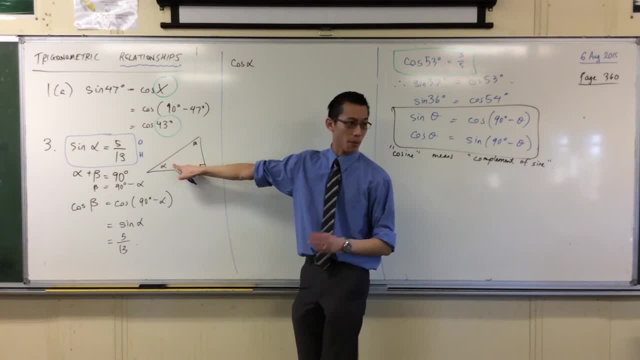 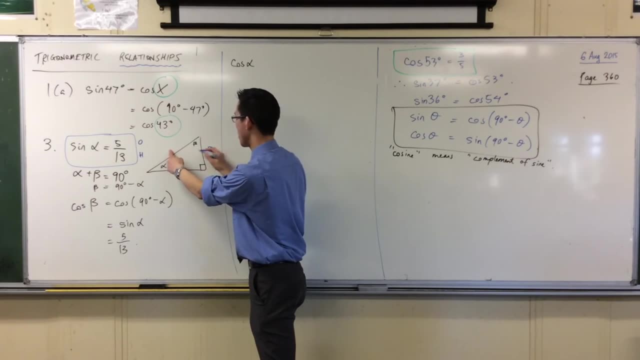 Opposite over hypotenuse. So if that's where I'm looking from, if that's my viewpoint, my perspective, then opposite and hypotenuse are these guys. So that should be the ratio 5, 13.. 5 and 13.. 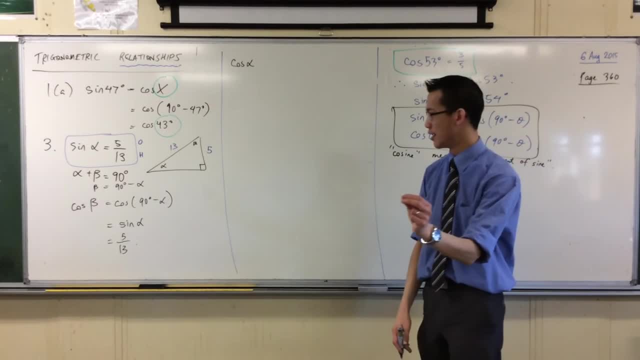 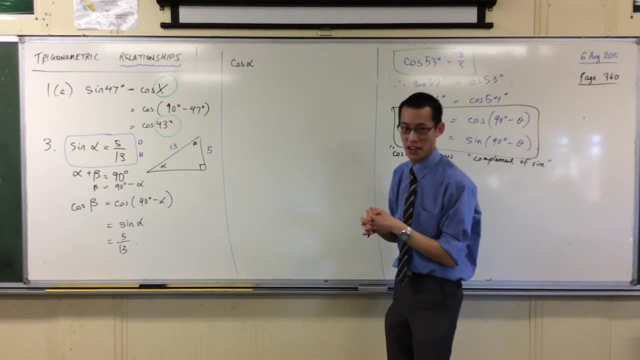 Now, the reason why that's useful is because this is a right angle triangle. We've been doing trig with right angle triangles, but go all the way back to like 7 and 8.. What else do you know about right angle triangles? 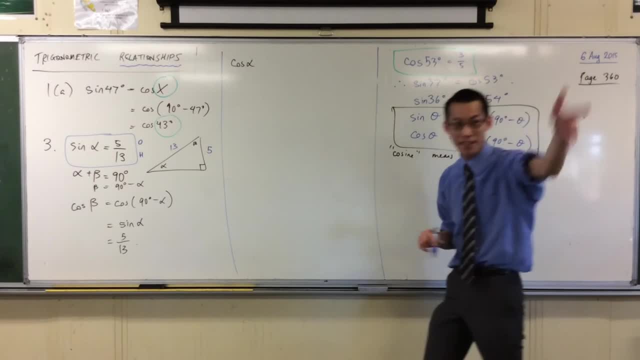 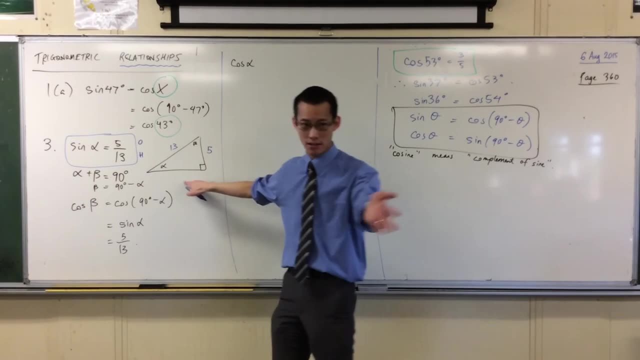 Think old Greek guy with an awkward name. Yeah, Pythagoras' theorem. right, If I know 5 and 13,. if I know two sides, I can work out the last side. Now you can go ahead, You can reach for your calculator. 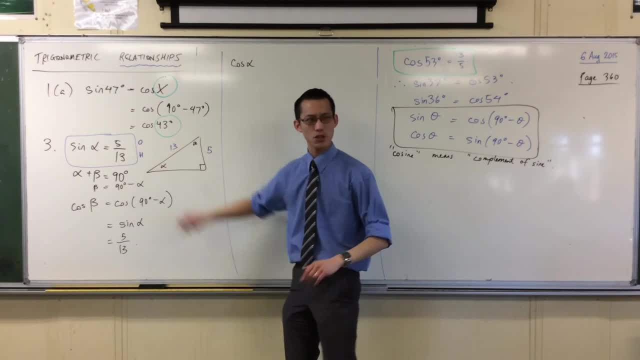 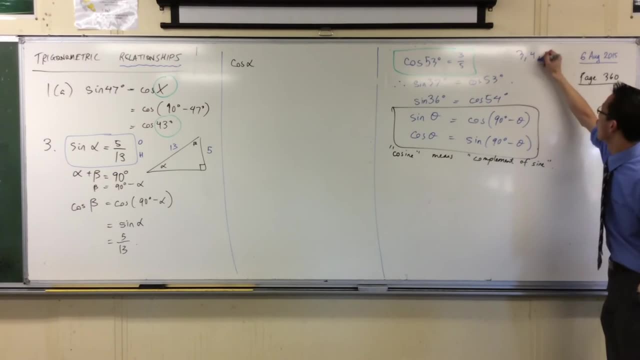 This squared plus this squared equals this squared. But you sort of want to get to the point where you're thinking. I think I recognize this right. Like you know how I said, 3,, 4,, 5 is a very common right angle.